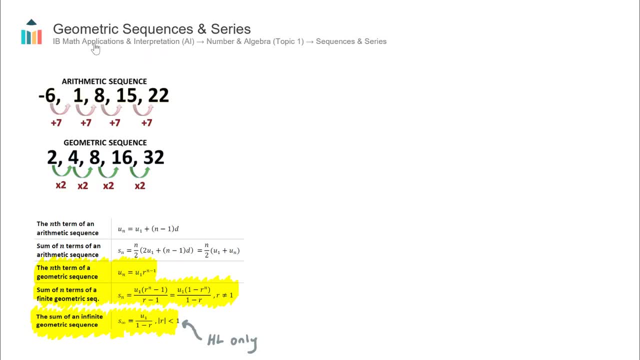 This video covers geometric sequences and series, an important concept found in IB Maths AI, Topic 1,: Number and Algebra. Now, there are two types of sequences that we encounter in the IB Maths AI course. They are arithmetic sequences and geometric sequences, which is the focus of 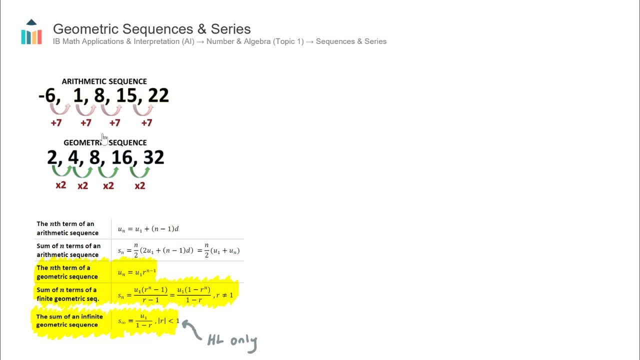 this video. Now just to recap the difference. an arithmetic sequence will either increase or decrease by a common difference. So, for example, in this sequence of numbers it is increasing by seven, each time an addition of seven, and we call that a common difference of seven. 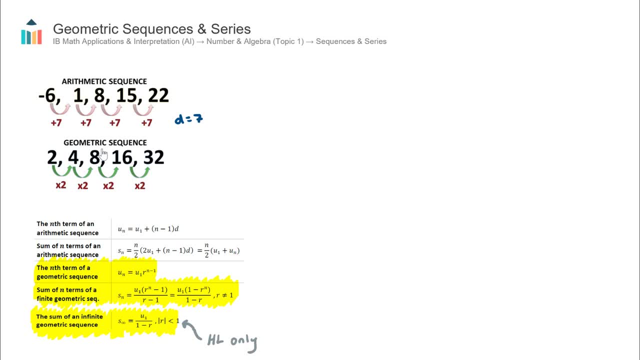 As opposed to geometric sequences, we'll either increase or decrease by a common ratio. So for example, in this sequence it's going up by a multiplication factor or a ratio of two each time. So we call that a common ratio of two. 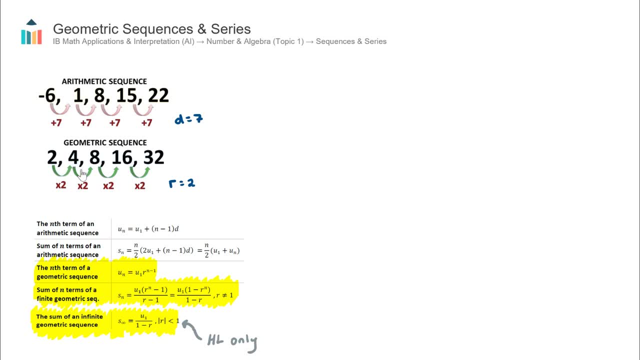 Now a little bit more notation that we need to know. The labels that we give to term values is U. So, for example, this first term we call U1,, the second term we will call U2,, third term U3, and so on and so on. So that's the notation that we need to know. First term, second term. 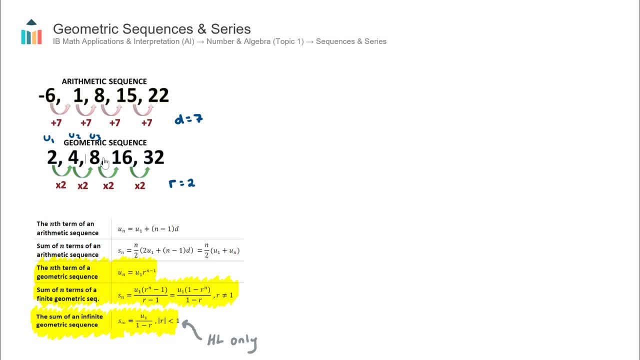 third term, common ratio. And then also, if we wanted to find some sort of term in the difference- and let's say we weren't sure on that term- we would call that U? n, So that would be the nth term in the sequence. 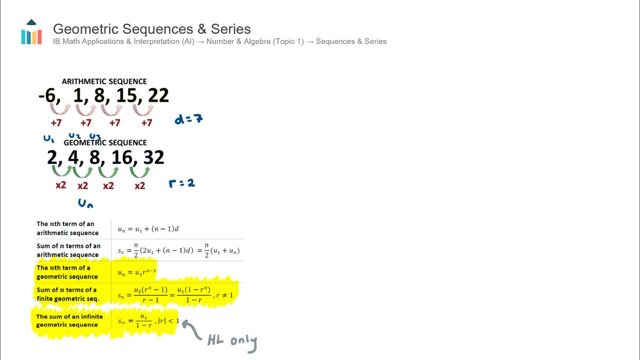 Now let's go through a few more examples of geometric sequences, because it's important to visualize them when we start to encounter negative ratios and also fractional ratios. So I want to go through three more. The first is this one: here, Let's say, we have a first term of five, a second term of negative 25,, a third term of 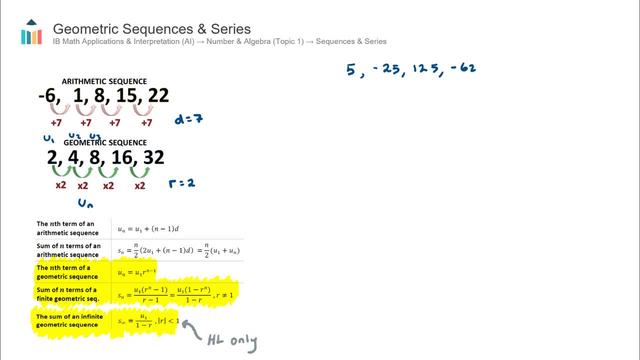 125,, a fourth term of negative 25, and a fifth term of negative 625,. dot, dot dot. So this sequence continues on indefinitely. Well, we know that our first term, U1, is five. Our second term, negative 25, is negative 25.. 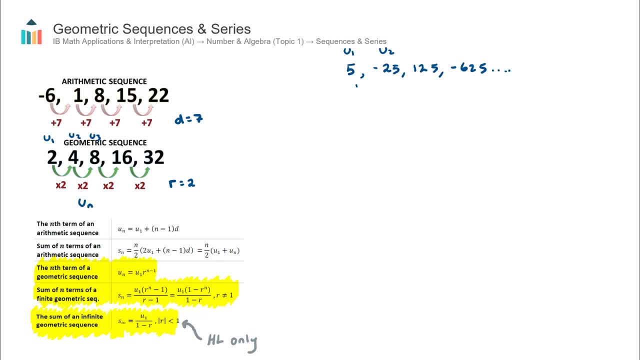 But what I'm interested in talking about is what's our common ratio here? How do I get from five to negative 25?? Well, you could either do this in your head, but one way to find out what it is is using this formula here. 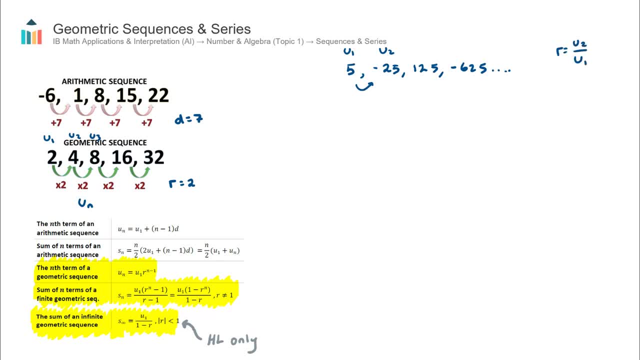 The common ratio is the second term divided by the first term, which is also equal to the third term divided by the second term, and so on and so on. So in this case here, negative 25 divided by five, and you can test this in your calculator if you like, but that will be. 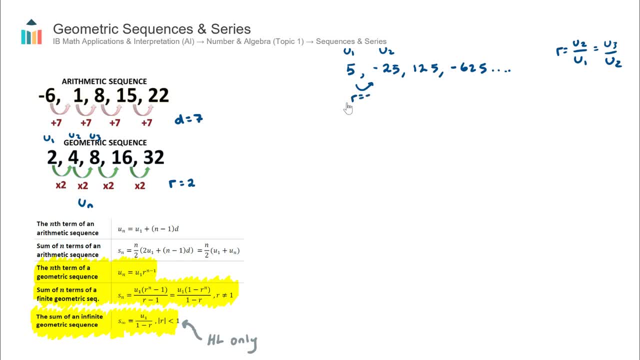 negative five. sorry. So my common ratio is actually negative five, and that holds up for this sequence: Negative five, negative five. So you'll start to notice here that if we have a negative common ratio, the term values will switch between positive and negative numbers, because a positive number multiplied by a negative is a negative and negative number multiplied by a negative is a positive, and so on and so on. 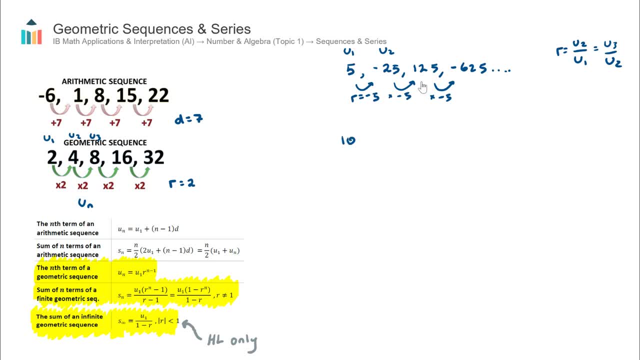 Okay, another type of geometric sequence is this one here: 100, 50,, 25.. 12.5,, so on and so on. Now, what's the common ratio in this sequence? Well, how do we get from 100 to 50?? 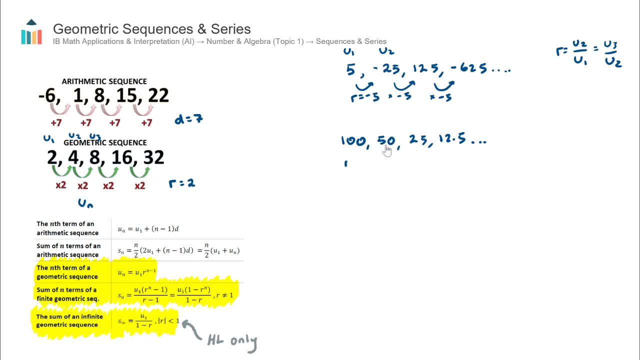 Well, we divide by two or another way to write. that would actually be multiplied by a half, and that's the same for this and the same for this. So our common ratio here is actually a half. So when we have a fractional common ratio, the terms will decrease over time. 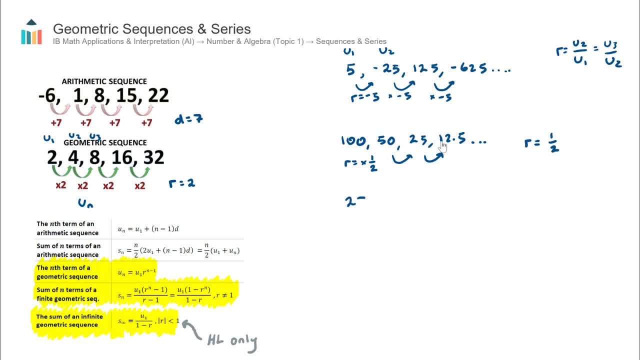 Now, one more that I want to go through is this one here: 27, negative nine, three negative one and then one on three. Well, this is kind of a combination of the previous two. I'm both switching between positive and negative numbers, and it's also going down. 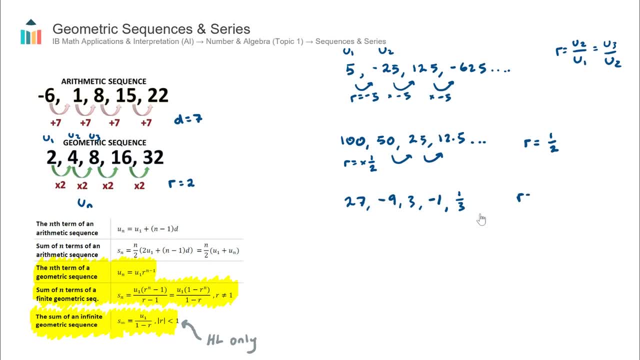 And if you were to work this through, you would notice that the common ratio would actually be: it's a negative number because we're switching between the two And it's also going to be a fractional number and it actually results in being negative. one on three. 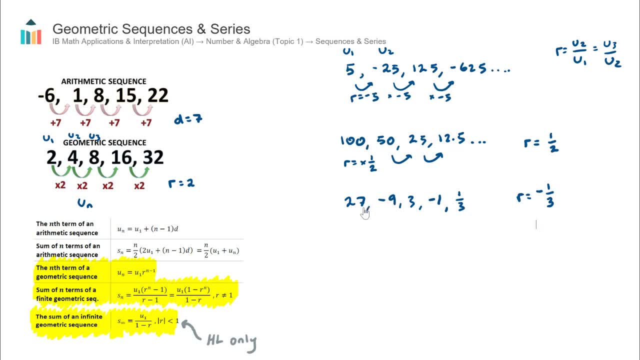 And if you wanted to test that you could actually do. the second term divided by the first term, That would be negative nine on 27, which is negative one on three. Okay, now that we have talked through a few different examples of geometric sequences, 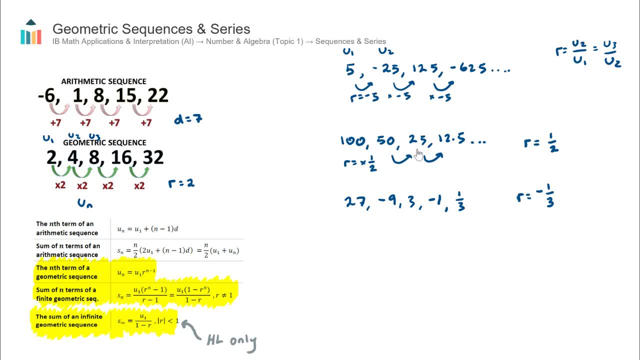 let's look at the formulas given to us in our IB Maths AI formula booklet and go through a couple of examples. So there are three formulas given: The first which most relate to the, the SL and HL course, and the third one here is just HL only. 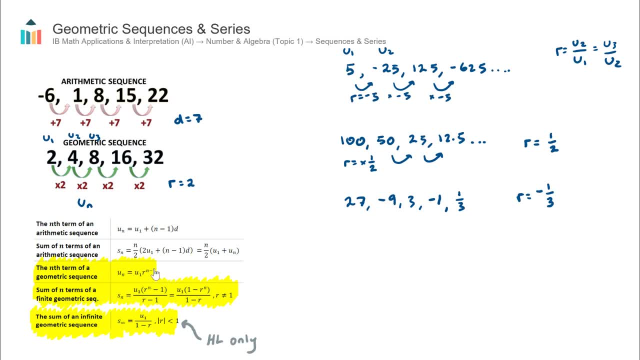 So let's work through these first two. The first formula here is very useful to find some sort of term in the future. So, for example, if I was to use this sequence here: now we know the first, second, third, fourth and fifth term. 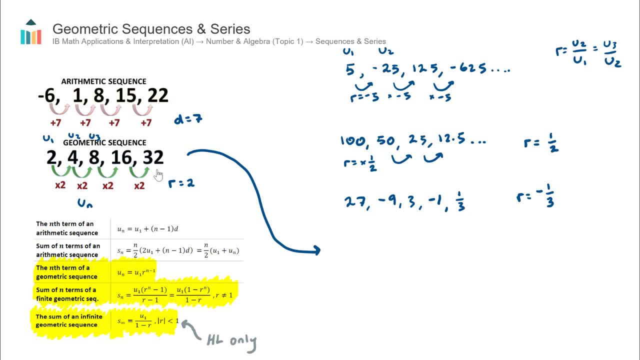 but what if I was to ask you to find the eighth term in the sequence? So what if I was to find U8?? Now, because these numbers are getting quite big quite fast, that might be mentally challenging. So fortunately we have a formula here to quickly find that result. 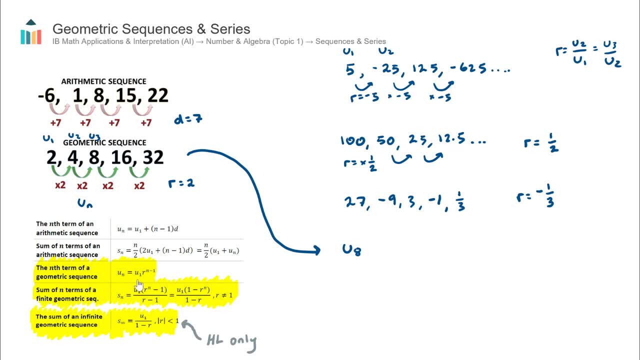 So that formula is equal to the first term, U1, which is two multiplied by the common ratio to the power of n. take one, so our common ratio is two to the power of. now the n is the term value that we're trying to find, which in our case is: 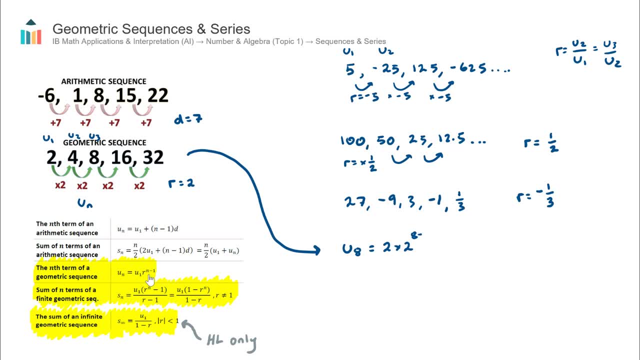 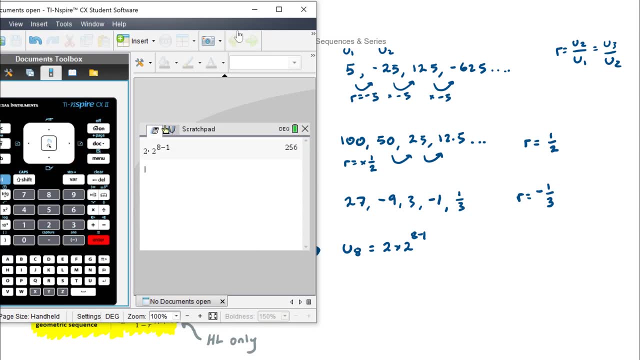 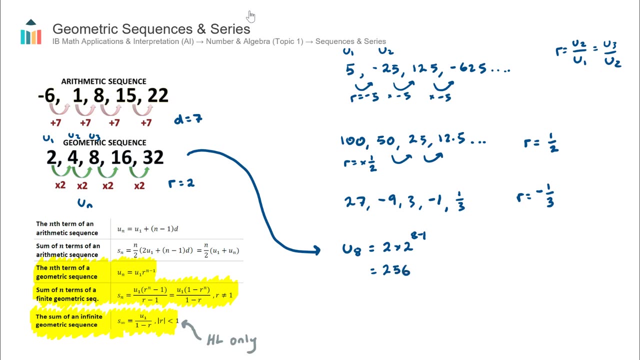 the eighth term. so this will be to the power of eight subtract one. Now we can use our calculator to find out that result, and that is 256.. So the eighth term in our geometric sequence here is 256.. Okay, so that covers this first formula here. 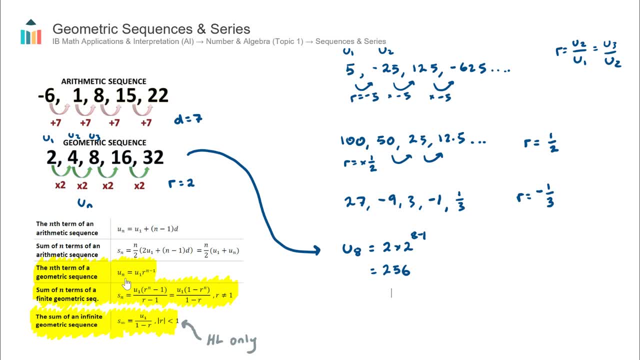 which is finding the nth term in a of a geometric sequence, so some sort of term value in the future. The next formula. there's actually two of them, but I'll talk through it later through each one. These both help us to find the sum of a certain number of terms in a sequence. 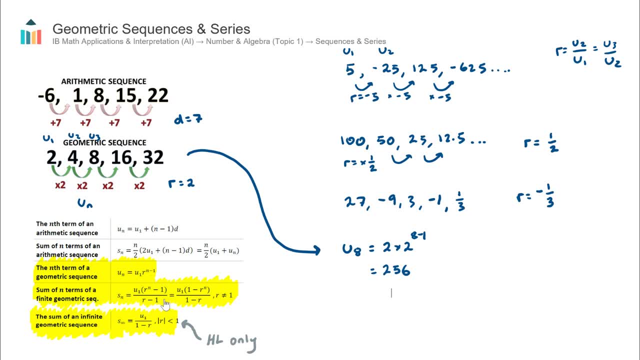 and that's what's called a series. So a series is a sum of terms in a sequence. So, again using this example, what if we wanted to find the sum of the first ten terms? So that would be adding up two plus four plus eight plus sixteen plus thirty-two. 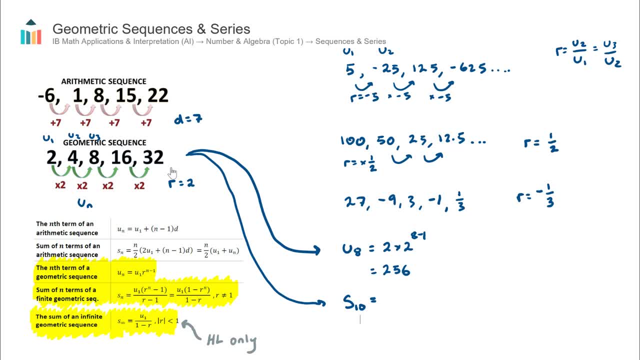 and then also finding the sixth term, seventh term, eighth term, etc. And then adding them all up together. Doing that by hand would be quite difficult and quite time-consuming. Fortunately, we have a formula here to do that quite quickly Now. there are two formulas listed here You can actually use either. 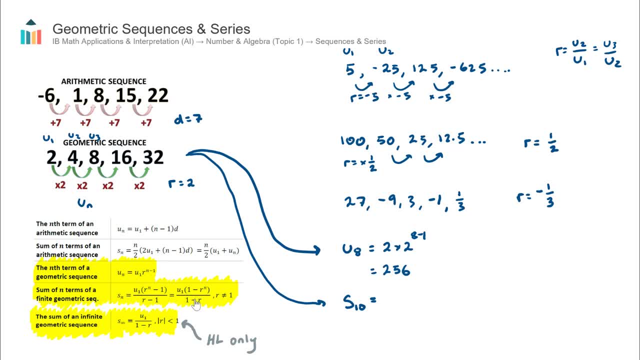 I tend to only use the left-hand one, The right-hand one. the working just becomes a little bit cleaner if the common ratio is less than one. So between, say, negative one and one, the working here will be a little bit cleaner. 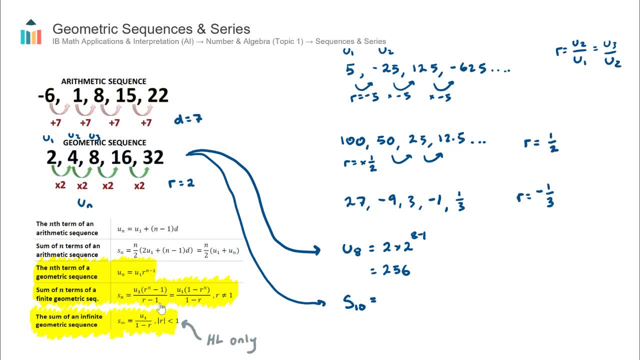 But if you just use the left-hand one, you would get the correct answer. You just have a few negatives on both the top and the bottom, Okay, so let's use this left-hand one here. The formula is equal to the on the numerator, the top of the fraction. 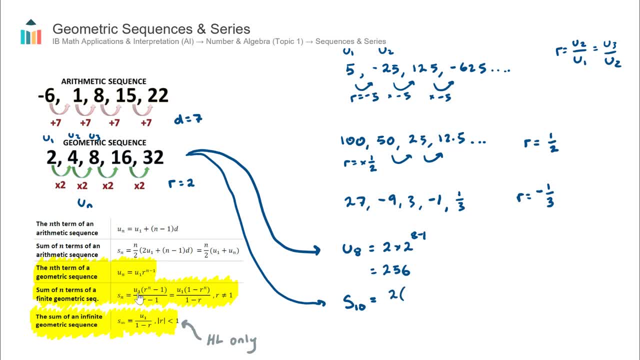 it'll be the first term, which is two Multiplied by our common ratio, which is two to the power of n, which is the sum of the first ten terms. So that'll be ten Subtract one, all divided by our common ratio, subtract one. Now common ratio is two, so two subtract one. Now we can use our 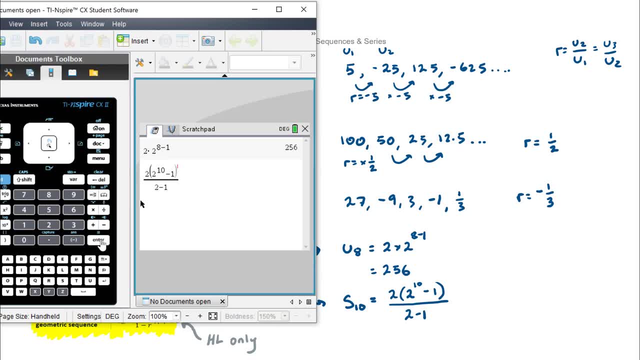 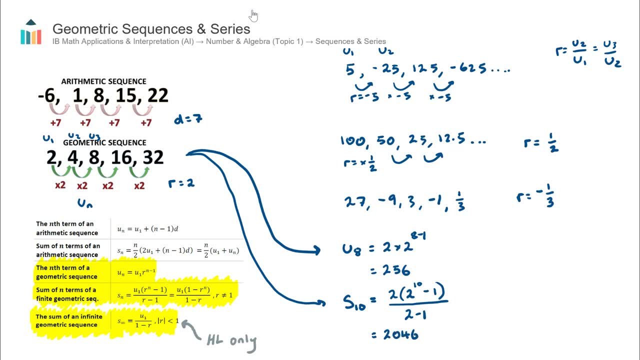 calculator from there to find that result. I've entered it there and that gets an answer of 2046.. So if we were to add the first 10 terms in this sequence, we would get an answer of 2046.. Now if you're an IB Maths, AISL student, feel free to stop the video there, because that concludes. 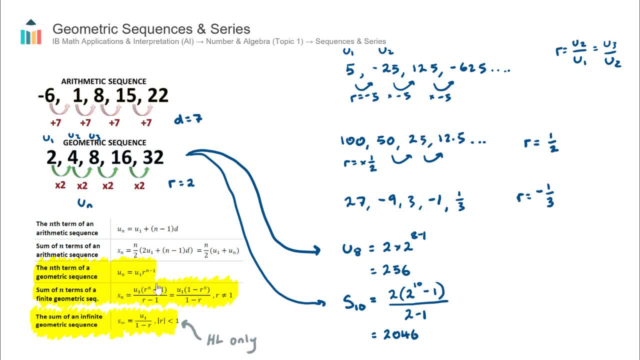 the content for your course, But if you're a HL student, let's just continue on and cover this last formula here: the sum of an infinite geometric sequence. Now, this formula here is useful if the common ratio is less than one. So these two examples here are examples of that. 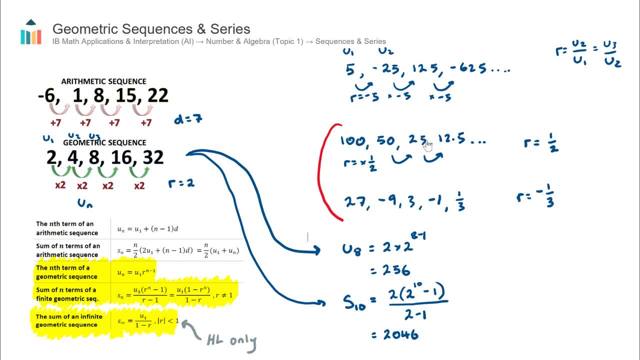 Now you can see here- let's focus on this first sequence of numbers- here- The term values are getting smaller and smaller. So therefore, eventually the terms will get so small that the total sum actually hits a limit. It doesn't get bigger and bigger and eventually.